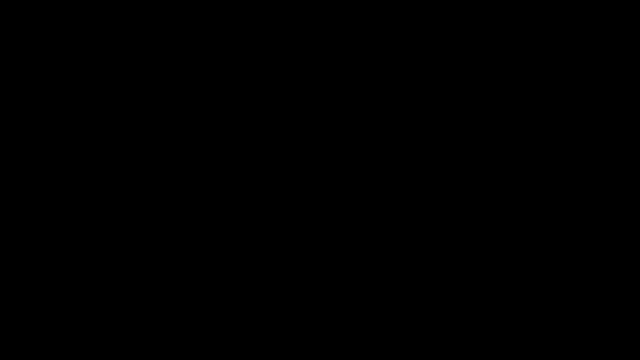 In this video, we're going to focus on solving differential equations by means of separating variables. So let's start with this example problem: dy dx is equal to x squared divided by y squared. Now in this problem, what we need to do is separate the variables. 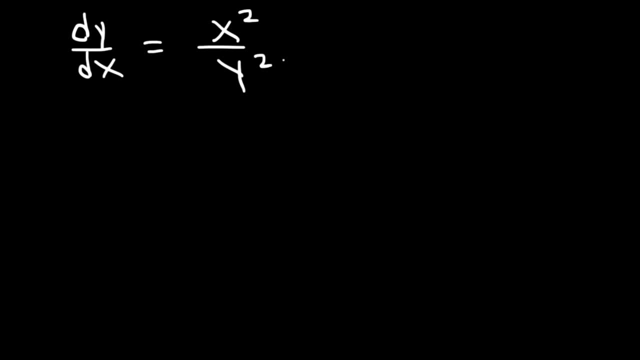 On one side, we only want to have y variables And on the other side of the equation, we only want to have x variables. So since we have a fraction separated by an equal sign, let's cross multiply dy times. y squared is simply y squared dy. 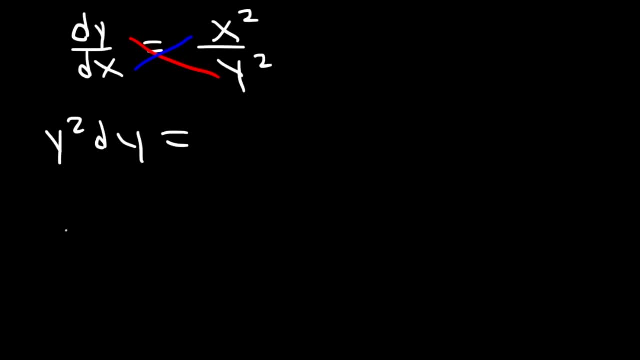 And on the other side it's going to be x squared dx. Now that we've separated the variables, we can integrate both sides of the function. The antiderivative of y squared is y cubed divided by 3.. The antiderivative of x squared 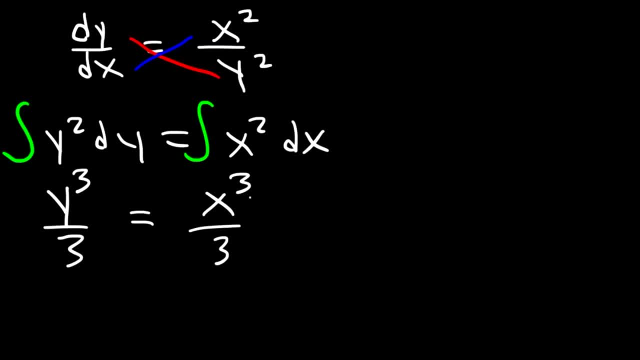 The antiderivative of x squared is y cubed divided by 3.. The antiderivative of x squared is x cubed divided by 3.. And on one side of the equation we need to add a constant c. So now let's get y by itself. 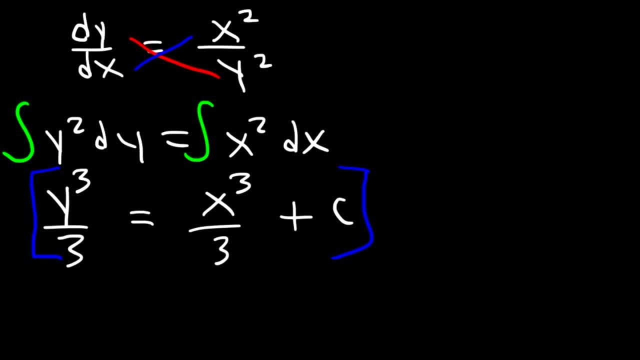 So let's multiply both sides of the equation by 3.. So it's going to be: y cubed is equal to x cubed plus 3c. Now 3c is a constant, So we can just write c for the total sum of all constants. 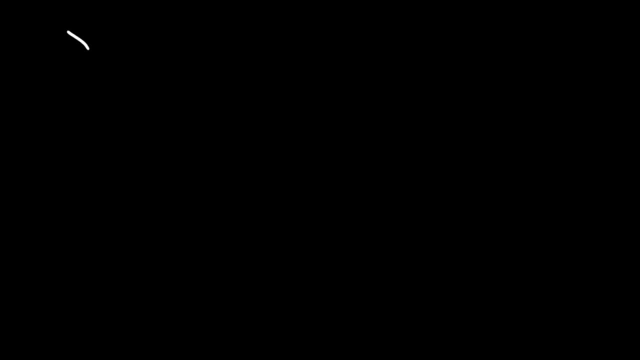 So you can rewrite this as y cubed is equal to x cubed plus c, And so this is the answer. Now, if you want to, you can take the cube root of both sides and simplify it further. So y is equal to the cube root of x cubed plus c. 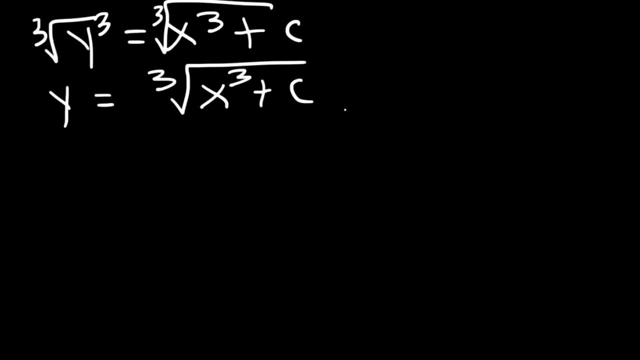 So this is the general solution. Now let's say, if we want to find a particular solution, If we're given an initial condition, let's say y of 1. Is equal to 2.. If you're given a point, an x and y value, you need to solve for c. 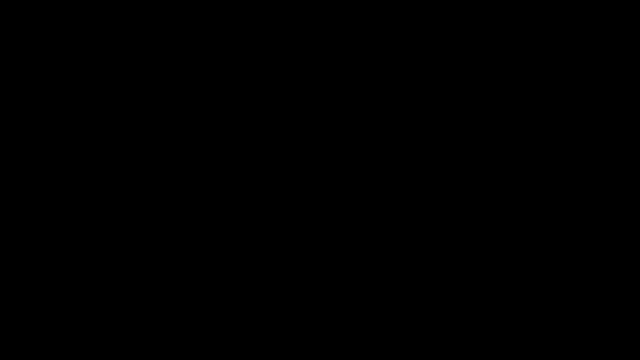 In this video, we're going to focus on solving differential equations by means of separating variables. So let's start with this example problem: dy dx is equal to x squared divided by y squared. Now in this problem, what we need to do is separate the variables. 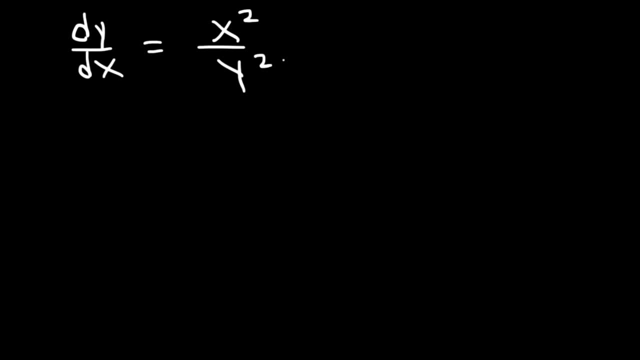 On one side, we only want to have y variables And on the other side of the equation, we only want to have x variables. So since we have a fraction separated by an equal sign, let's cross multiply dy times. y squared is simply y squared dy. 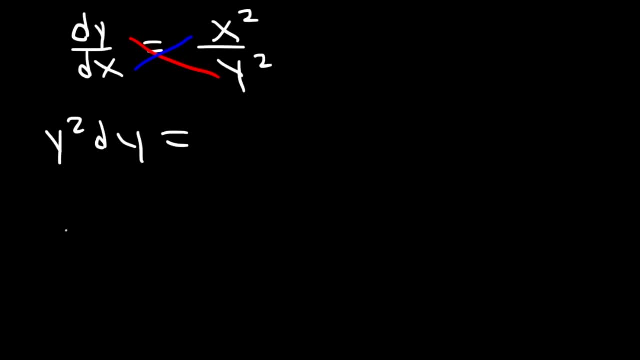 And on the other side it's going to be x squared dx. Now that we've separated the variables, we can integrate both sides of the function. The antiderivative of y squared is y cubed divided by 3.. The antiderivative of x squared 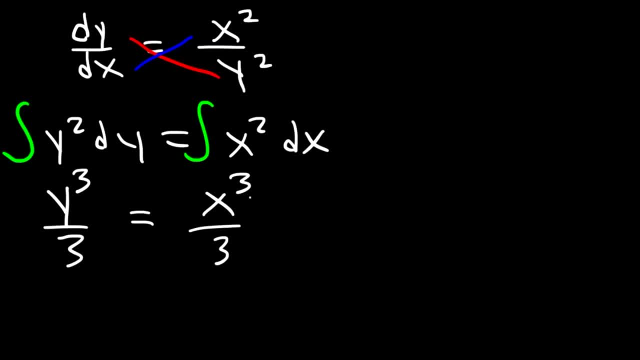 The antiderivative of x squared is y cubed divided by 3.. The antiderivative of x squared is x cubed divided by 3.. And on one side of the equation we need to add a constant c. So now let's get y by itself. 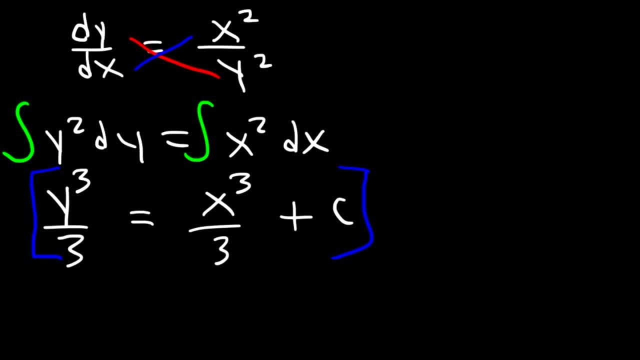 So let's multiply both sides of the equation by 3.. So it's going to be: y cubed is equal to x cubed plus 3c. Now 3c is a constant, So we can just write c for the total sum of all constants. 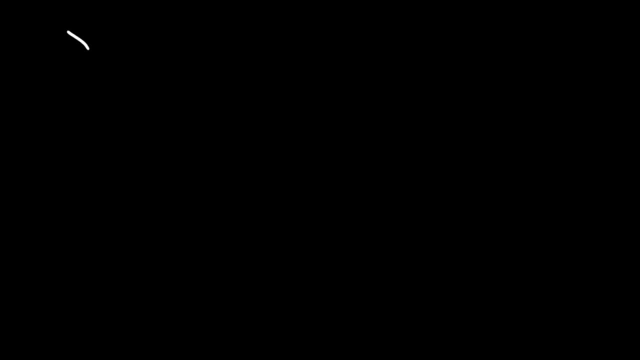 So you can rewrite this as y cubed is equal to x cubed plus c, And so this is the answer. Now, if you want to, you can take the cube root of both sides and simplify it further. So y is equal to the cube root of x cubed plus c. 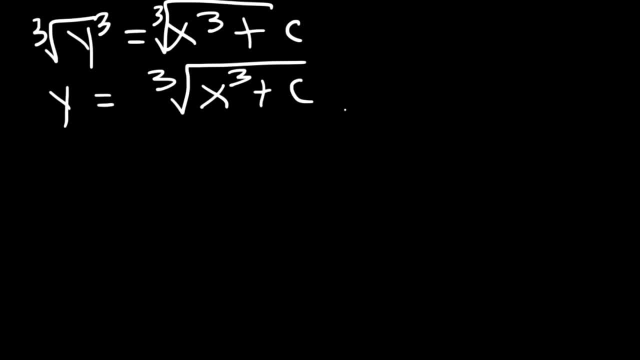 So this is the general solution. Now let's say, if we want to find a particular solution, If we're given an initial condition, let's say y of 1. Is equal to 2.. If you're given a point, an x and y value, you need to solve for c. 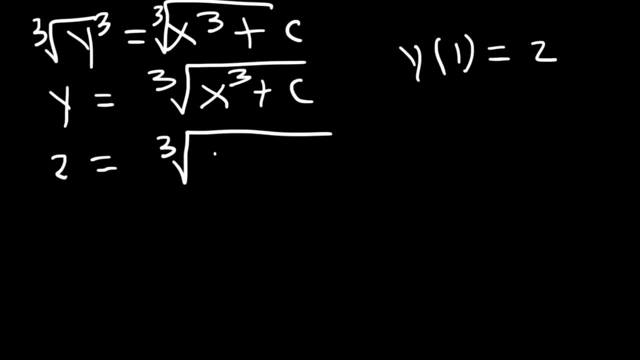 y is equal to 2. And x is equal to 1.. So in order to get c by itself, we need to raise both sides to the third power. 2 to the third is equal to 8.. The cube of a cube root cancels and it's just going to be 1 plus c. 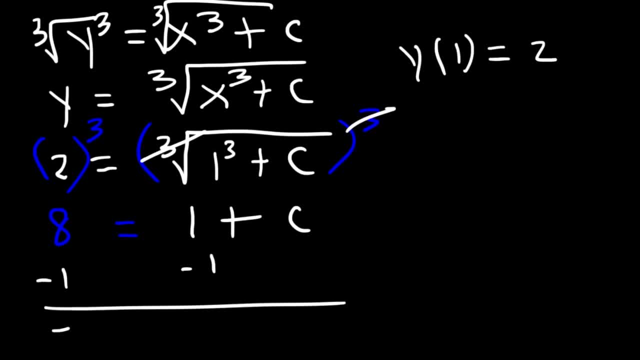 So we can see that 7 is equal to c. So the particular solution is: y is equal to the cube root of x, cubed plus 7.. So this is the general solution and this is the particular solution, given the initial condition. 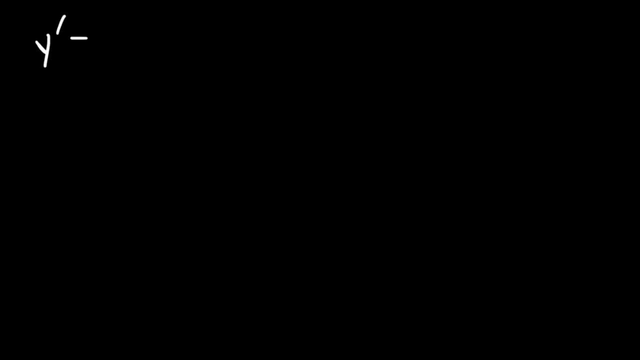 Let's work on another example. Let's say that y prime is equal to x times y. Go ahead and pause the video and see if you can get this answer. And let's say that the initial condition is y is 0 is equal to 5.. 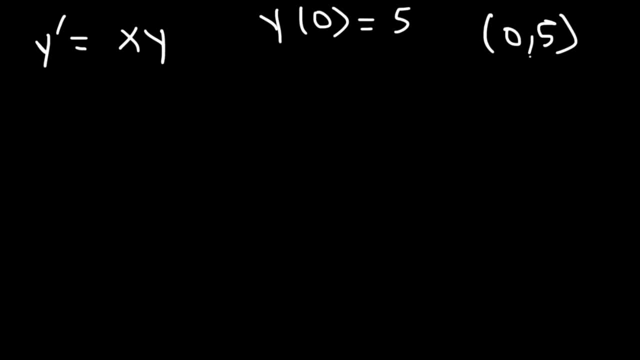 You can also view this as the point 0, comma 5.. x is 0 and y is 5.. So let's begin. y prime is the same as dy over dx, So we need to separate x and y And let's begin by multiplying both sides by dx. 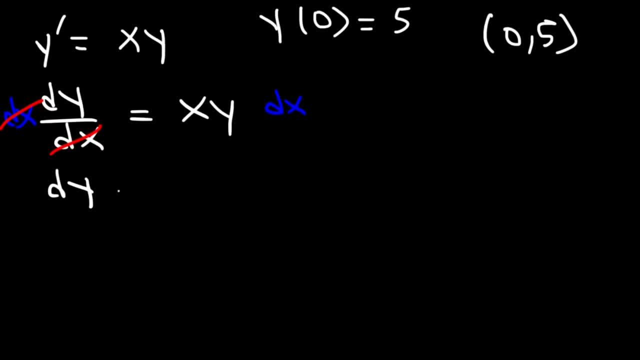 So therefore, dy is equal to xy dx. Now let's divide both sides by y. So on the left, what we have now is 1 over y dy, and this is equal to xdx. So now let's find the antiderivative of both sides. 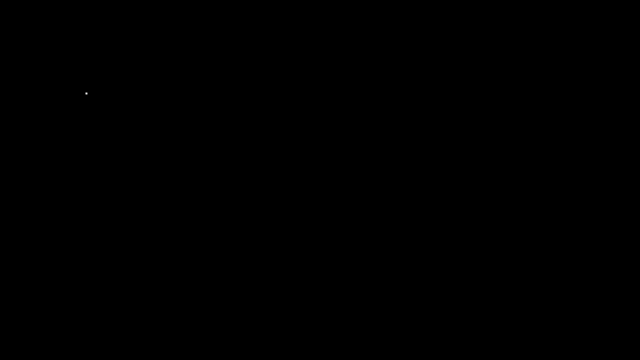 The antiderivative of both sides is y. So by dividing both sides by y We get to xy dy. So there we go of 1 over y is the natural log of y, or I'm just going to write it as l and y And the 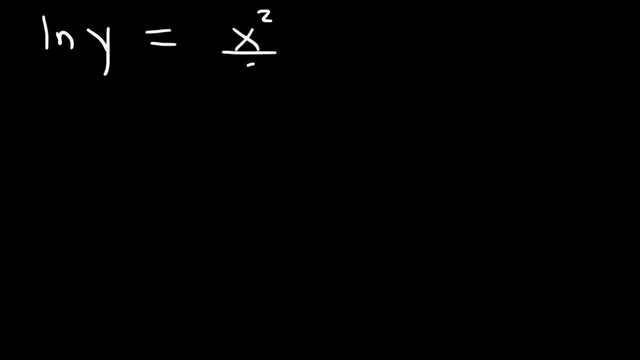 antiderivative of x is x squared over 2 plus c. So now, what do you think we should do at this point? At this point, what we can do is place both sides of the function on the exponents of e, If l and y is equal to x squared over 2 plus c. 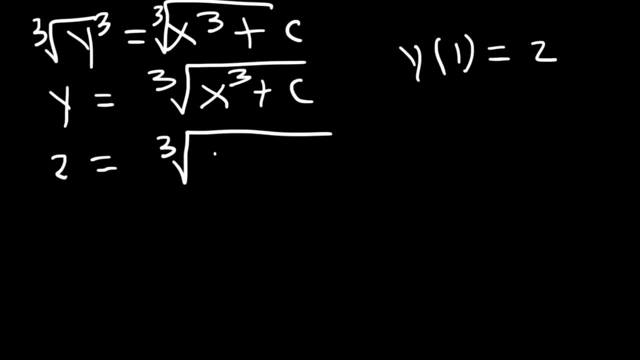 y is equal to 2, and x is equal to 1.. So in order to get c by itself, we need to raise both sides to the third power. 2 to the third is equal to 8.. The cube of a cube root cancels and it's just going to be 1 plus c. 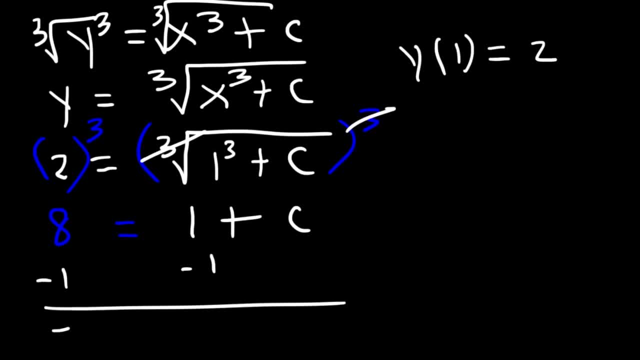 So we can see that 7 is equal to c. So the particular solution is: y is equal to the cube root of x, cubed plus 7.. So this is the general solution and this is the particular solution, given the initial condition. 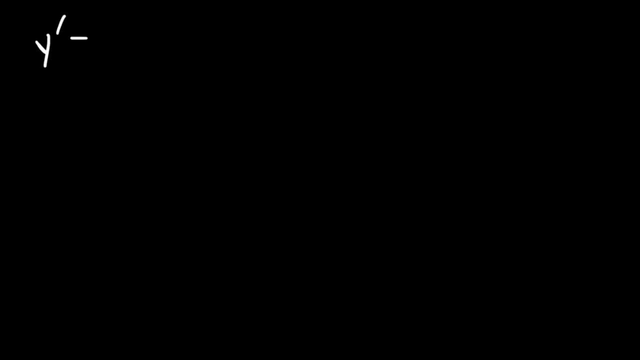 Let's work on another example. Let's say that y prime is equal to x times y. Go ahead and pause the video and see if you can get this answer. And let's say that the initial condition is y is 0 is equal to 5.. 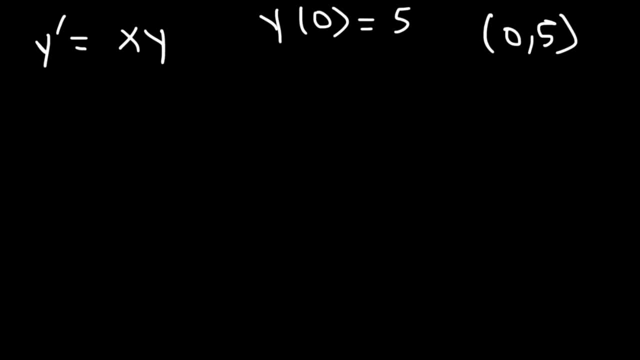 You can also view this as the point 0, comma 5.. x is 0 and y is 5.. So let's begin. y prime is the same as dy over dx, So we need to separate x and y And let's begin by multiplying both sides by dx. 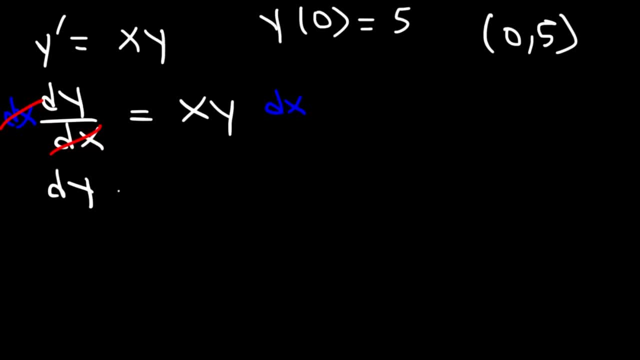 Therefore, dy is equal to xy dx. Now let's divide both sides by y. So on the left, what we have now is 1 over dy and x is equal to xяла, And this is equal to x- dx. So now let's find the antiderivative of both sides. 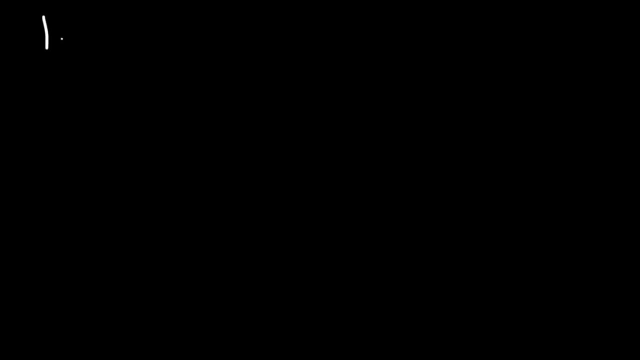 antiderivative of both sides. The antiderivative of 1 over Y is the natural log of Y, or I'm just going to write it as L and Y, And the antiderivative of X is X squared over 2 plus C. 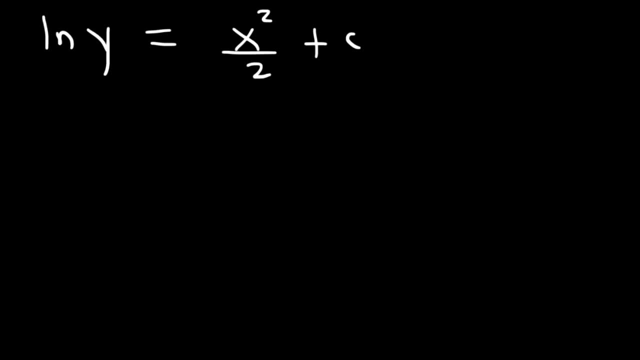 So now, what do you think we should do at this point? At this point, what we can do is place both sides of the function on the exponents of E. If L and Y is equal to X squared over 2 plus C, then E to the L and Y is equal to E one. 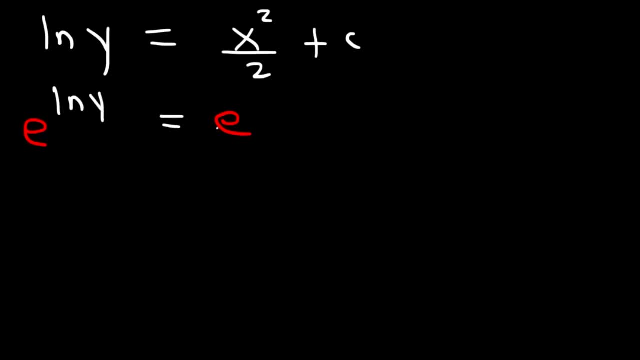 then e to the l and y is equal to e, one-half x squared plus c. Since the bases are the same, then the exponents are equal to each other. Now e to the l and y. notice that natural log always have a base e. These will cancel, and so 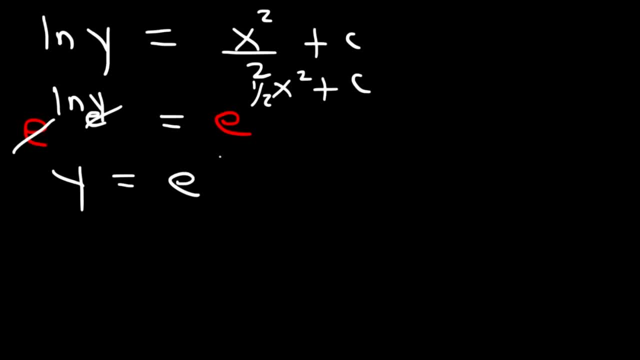 you just get y on the left side And that's equal to e raised to the one-half x squared plus c. Now how can we separate x squared and c? Now it's important to understand that x squared times x cubed is equal to x 2 plus 3, which is x to the fifth power, Whenever. 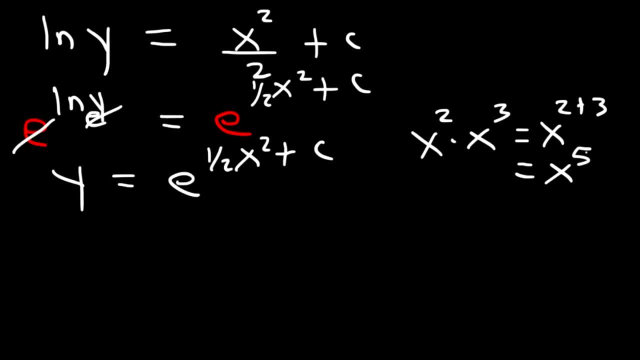 you multiply by common bases, you need to add exponents. So therefore the reverse is true. Let's say, if we have x raised to the 4 plus 7, we could separate 4 and 7 by rewriting as x to the fourth times x to the seventh, The same way as we did it here. So therefore we 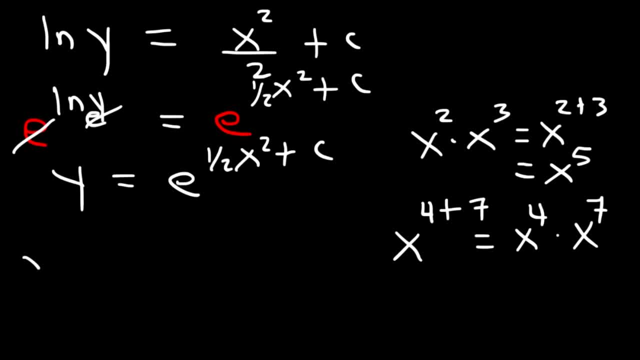 could separate the one-half x squared from c by means of multiplication. So this is e one-half x squared times e to the c. Now e raised to the c is a constant, So we could simply replace that with c. Therefore, the general solution is y is. 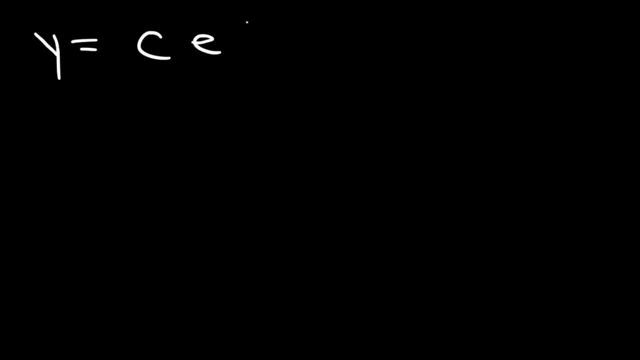 equal to c times e raised to the one-half x squared. Now the last thing that we need to do is find the particular solution. So we said that y of 0 is equal to 5.. So let's find the value of the constant c. So y is 5 and x is 0.. 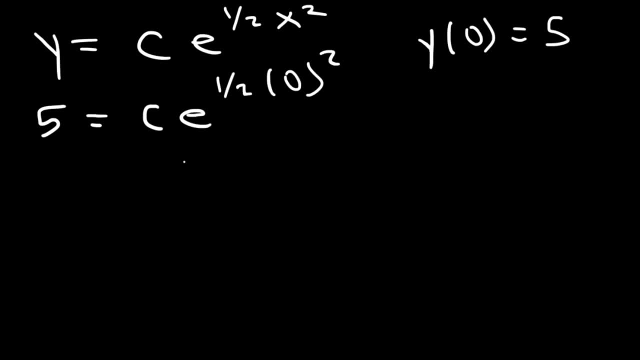 0 squared is 0.. Times a half, that's 0.. So what we have is e raised to the zero power. Anything raised to the zero power is equal to 1.. So therefore we could see that c is equal to 5.. So the particular solution is 5e raised to the one-half x squared, And so: 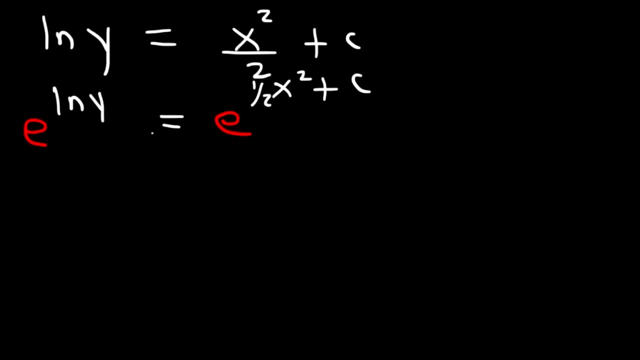 half X squared plus C. Since the bases are the same, then the exponents are equal to each other. Now E to the L and Y. notice that natural log always have a base E. these will cancel, and so you just get Y on the left side. 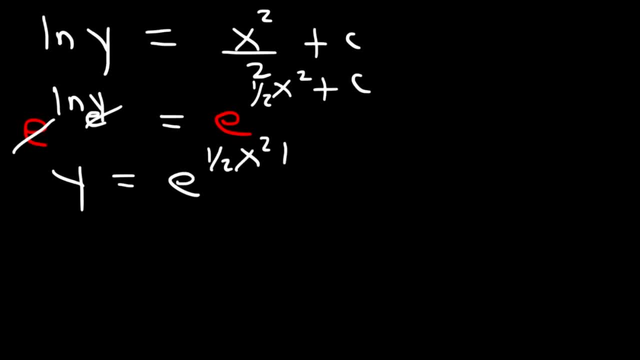 And that's equal to E raised to the one half X squared plus C. Now how can we separate X squared and C? Now it's important to understand that X squared times X cubed is equal to X 2 plus 3, which 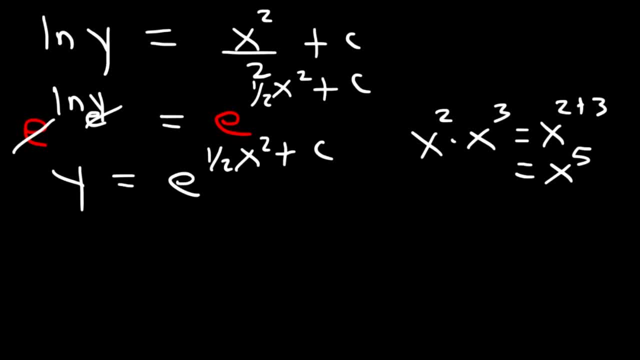 is X to the 5th power. Whenever you multiply by common bases, you need to add exponents. So therefore the reverse is true. Let's say, if we have X raised to the 4 plus 7.. X to the 4 plus 7.. 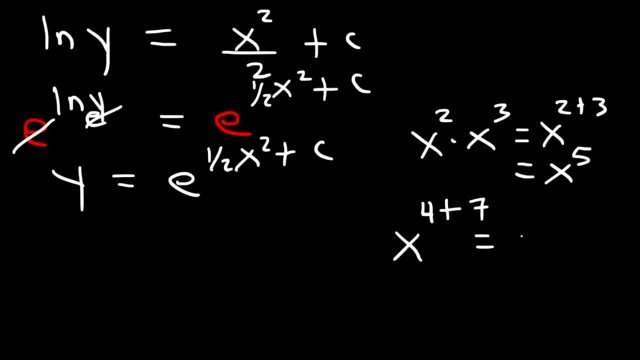 X to the 4 plus 7.. X to the 4 plus 7.. We could separate 4 and 7 by rewriting as X to the 4th times X to the 7th, The same way as we did it here. 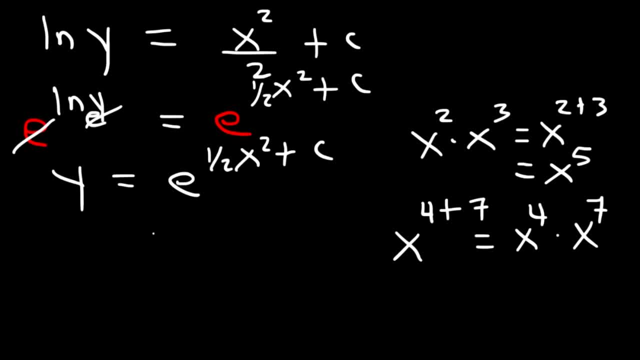 So therefore, we could separate the one half X squared from C by means of multiplication. So this is E, one half X squared times E to the C. Now, E raised to the C is a constant, so we could simply replace that with C. Therefore. 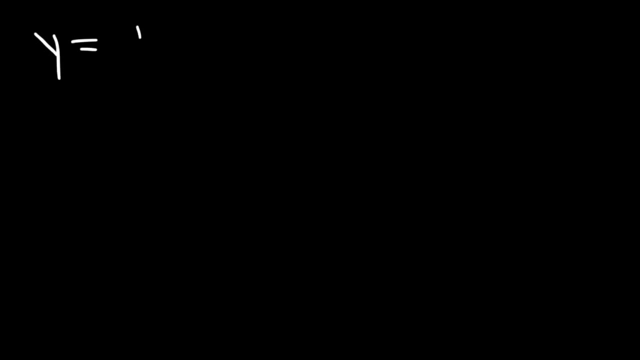 the general solution, Y is equal to C times E raised to the one half X squared. Now the last thing that we need to do is find the particular solution. So we said that Y of zero is equal to 5.. So let's find the value of the constant C. So Y is 5 and X is zero. 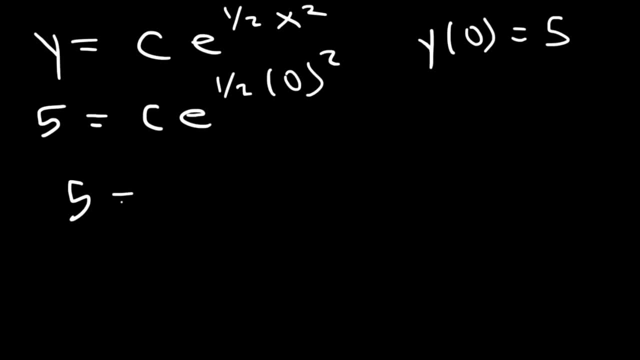 Zero squared is zero times a half, that's zero. So what we have is E raised to the zero power. Anything raised to the zero power is equal to 1.. So therefore we could see that C is equal to 5.. So the particular solution is 5 E raised to the one half X squared. 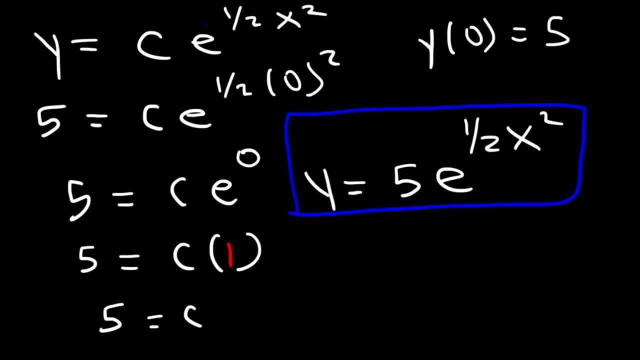 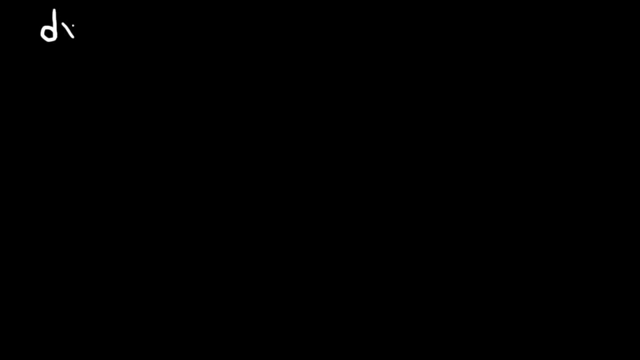 And so that's the answer to this problem, And here is the general solution. Here's another problem for you. Let's say that DY divided by DX, DX is equal to Y squared plus 1.. And let's say that you're given an initial condition. 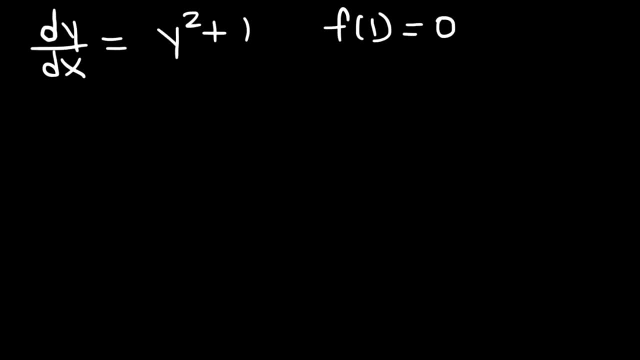 F of 1 is equal to zero, Or rather Y of 1 is equal to zero. So go ahead and find the general solution and the particular solution to this differential equation. So feel free to pause the video and work on this example. Now let's begin. 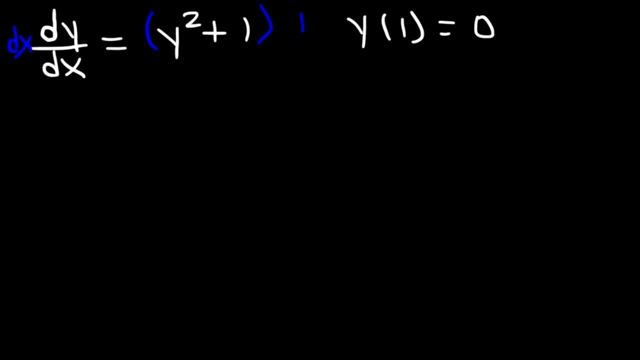 Let's start by multiplying both sides by DX. So what we now have is: DY is equal to Y squared plus 1 times DX. So we need to move the Y variable to the other side, And the best way to do that- to separate it from DX- is to divide both sides. 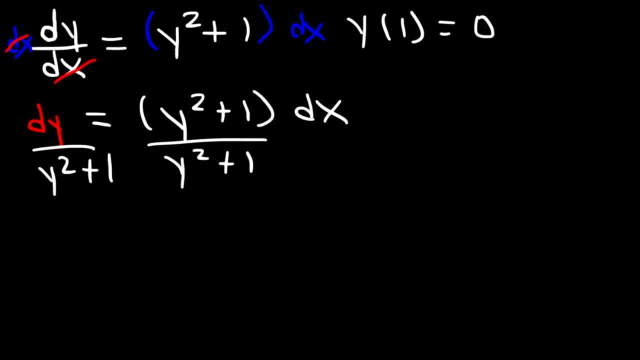 By Y squared plus 1.. Let's rewrite it as 1 over Y squared plus 1 times DY, and that's equal to DX. So now let's find the antiderivative of both sides. So what is the antiderivative of 1 over Y squared plus 1?? 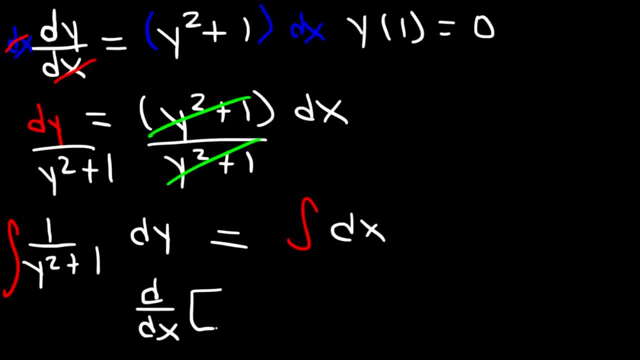 Well, It helps to know that the derivative of the inverse tangent of x is equal to 1 over 1 plus x squared. So this is going to be the antiderivative, I mean the antiderivative of 1 over y squared plus 1 is inverse tangent y. 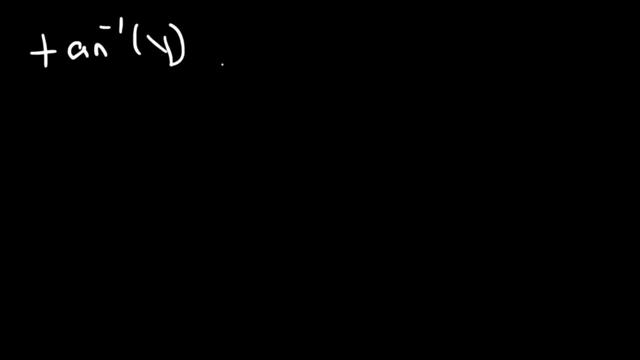 So that's what we're going to have on the left side. On the right side, the antiderivative of dx is simply 1x plus c, or just x plus c. Now what would you do at this point? What we need to do is take the tangent of both sides of the equation. 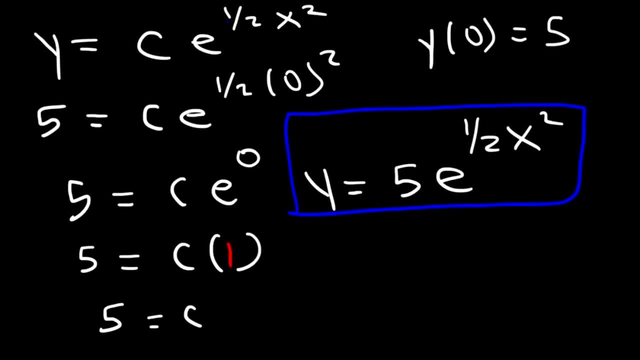 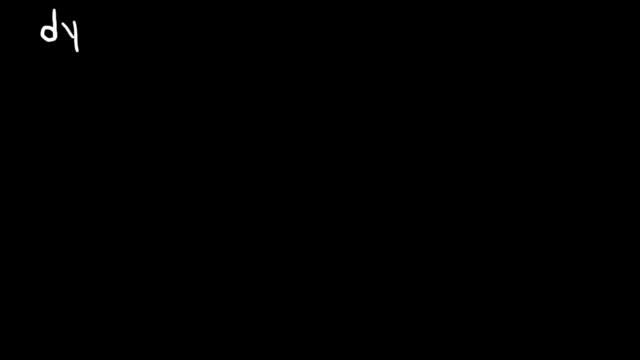 that's the answer to this problem And here is the general solution. Here's the answer to this problem And here is the general solution. Here's another problem for you. Let's say that dy divided by dx is equal to y squared plus 1.. And let's say that you're given an initial condition f of 1. 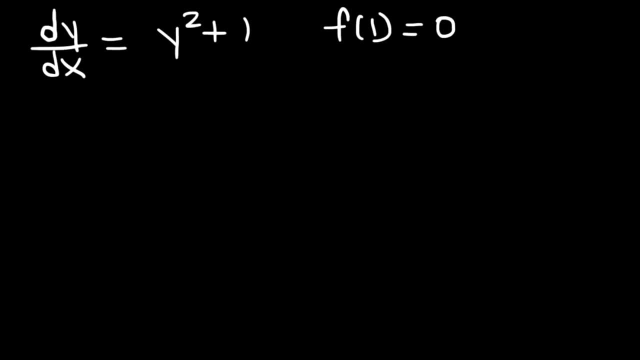 is equal to 0. Or rather, y of 1 is equal to 0. So go ahead and find the general solution and the particular solution to this differential equation. So feel free to pause the video and work on this example. Now let's begin. Let's start by multiplying both sides by Dx. So what we? 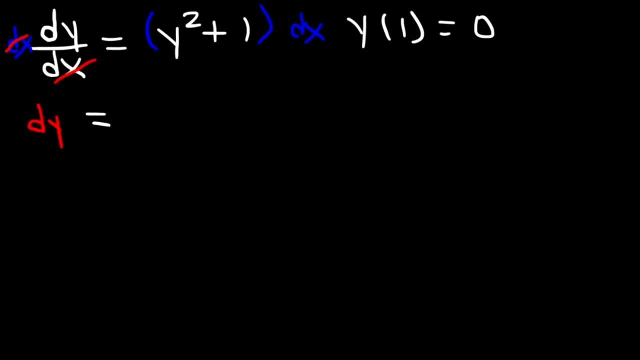 now have is: dy is equal to y squared plus 1 times dx. So we need to move the y variable to the other side, And the best way to do that, to separate it from dx, is to divide both sides by y squared plus 1.. 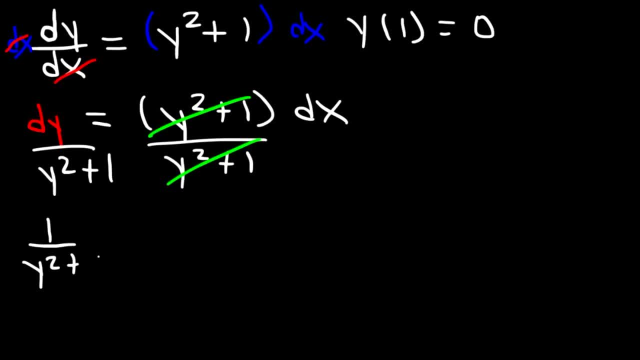 Let's rewrite it as 1 over y squared plus 1 times dy, and that's equal to dx. So now let's find the antiderivative of both sides. So what is the antiderivative of 1 over y squared plus 1?? 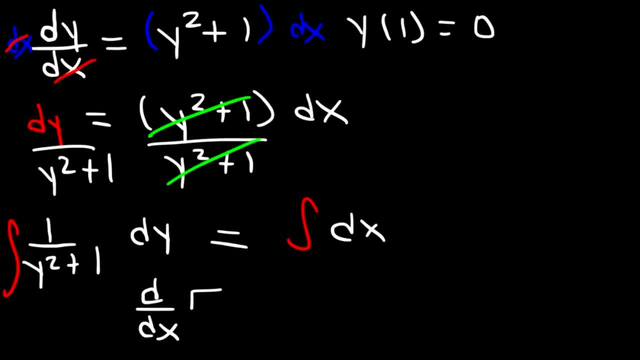 Well, it helps to know that the derivative of the inverse tangent of x is equal to 1 over 1 plus x squared. So this is going to be the antiderivative, I mean the antiderivative of 1 over y squared plus 1 is inverse tangent y. 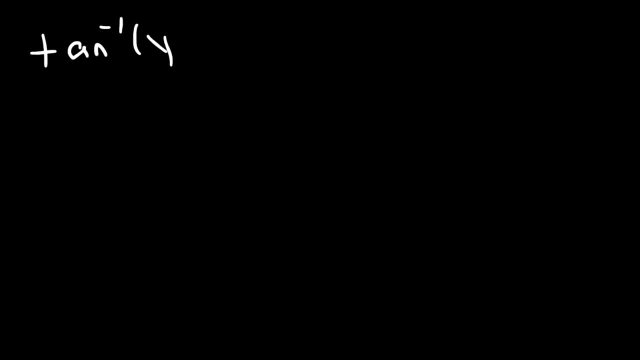 So that's what we're going to have on the left side. On the right side, the antiderivative of dx is simply 1x plus c, or just x plus c. Now what would you do at this point? What we need to do is take the tangent of both sides of the equation.